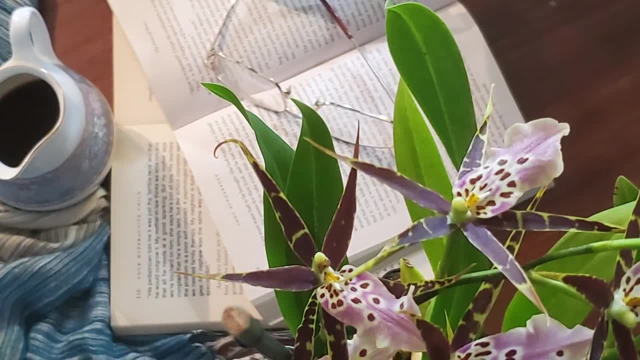 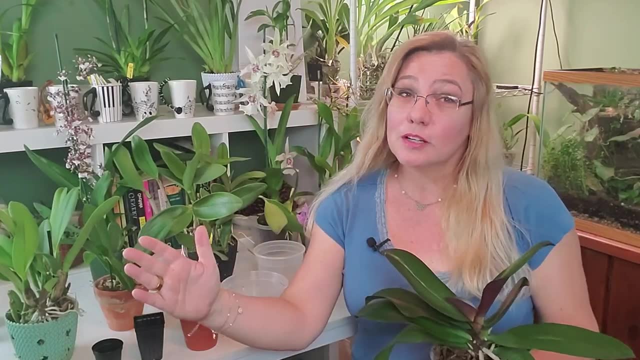 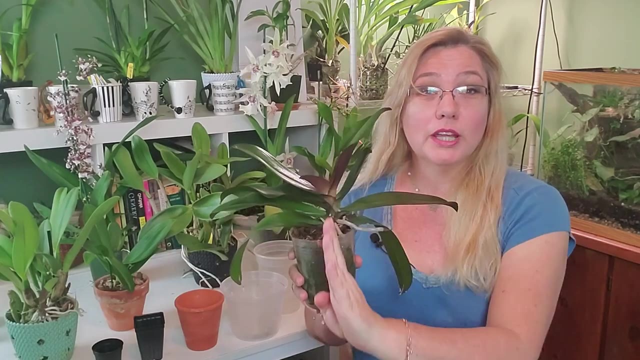 know how big of a pot to plant your orchid in. Well, that's going to depend on mainly one thing: What kind of orchid you have. First see if you have a monopodial orchid or a sympodial orchid. A monopodial orchid- mono means one. It's going to grow straight up. It's going to have one. 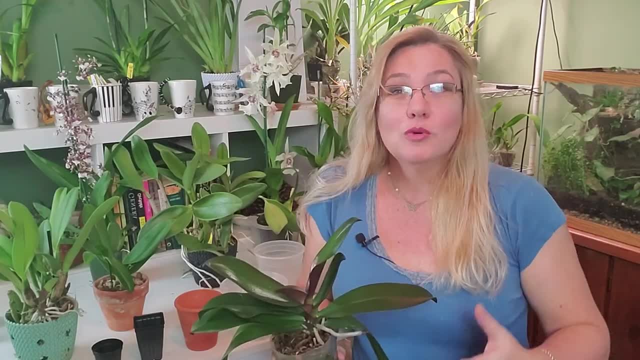 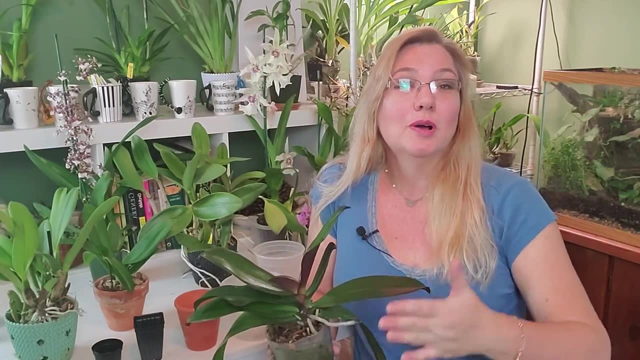 unique stem, which is like the Phalaenopsis orchid, which was probably the orchid that you bought first. So your monopodial orchid. you're going to want to pick a pot that is one inch larger, or 2.5 centimeters larger than that. 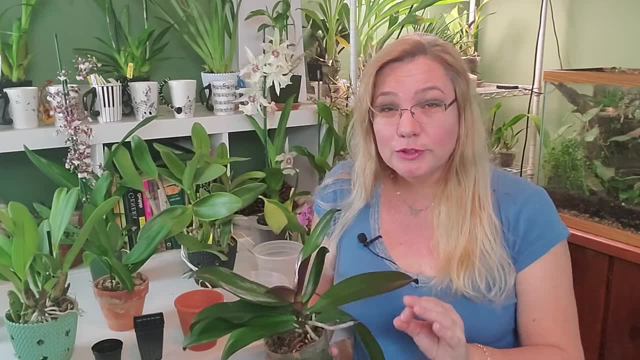 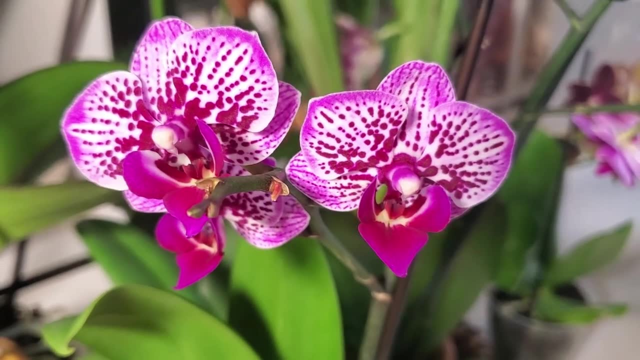 one that it's currently in. Usually, phalaenopsis we repot every two years, so that two year space is going to need a pot that's going to expand the roots in here for about an inch. Now a sympodial orchid means it has many. 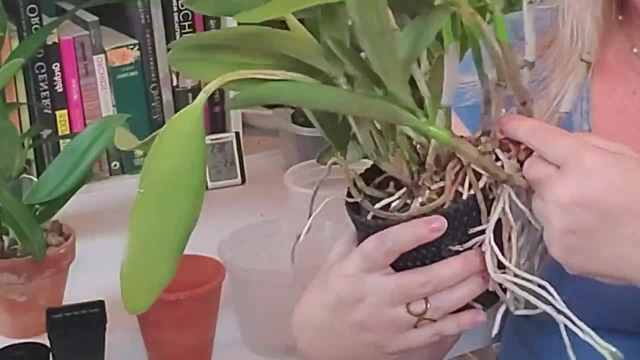 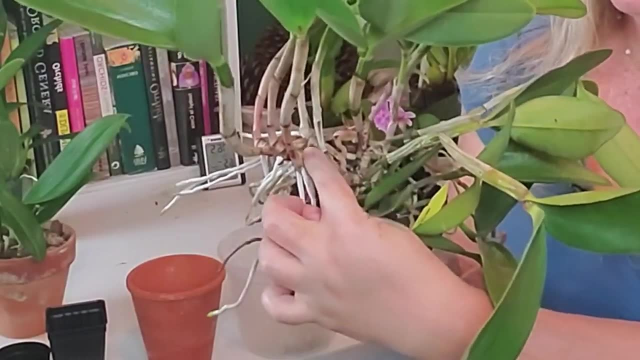 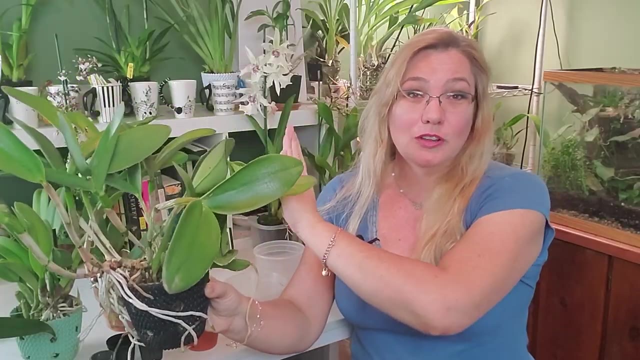 Instead of just one stem, it has many stems and it runs across a central rhizome that you can see right here. So this rhizome is going to grow and it grows out horizontally and from this horizontal rhizome then it's going to produce all those stems. So, sympodial orchids, you will need a larger pot. 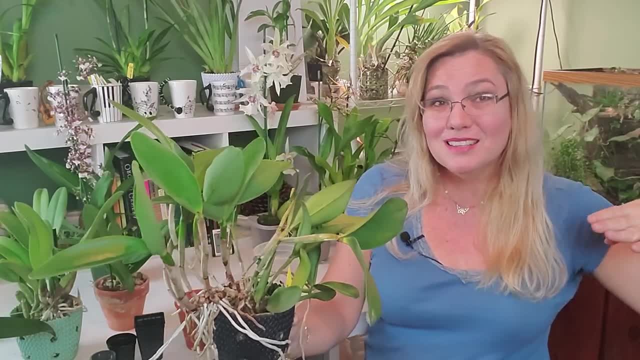 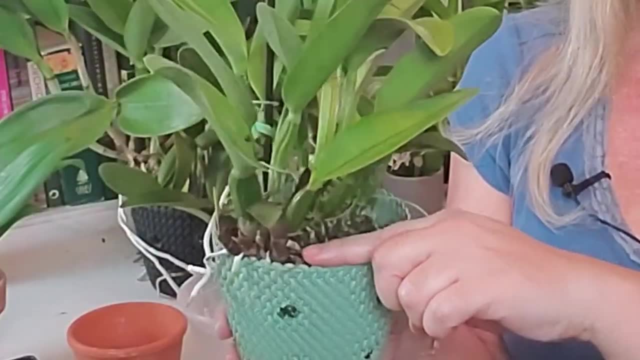 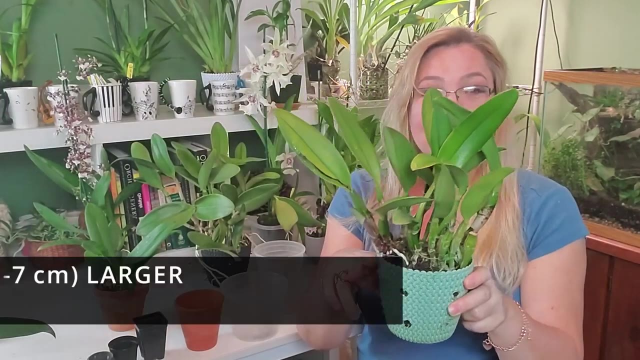 because during that two year time span it's going to travel out in all directions. This is also a new orchid: it's producing growth in both directions. so it's growing from this side and from this side, So I'll need to add both- a pot that can accommodate on both sides, unless I divide it, which I don't plan. 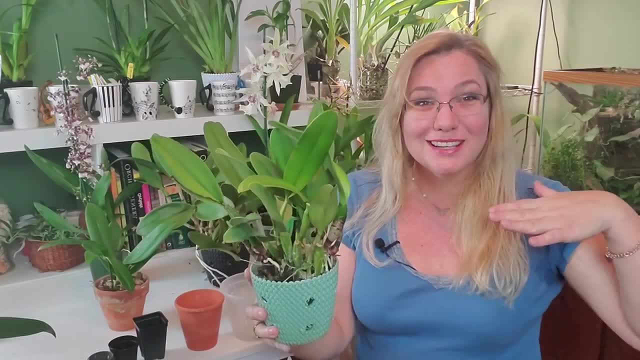 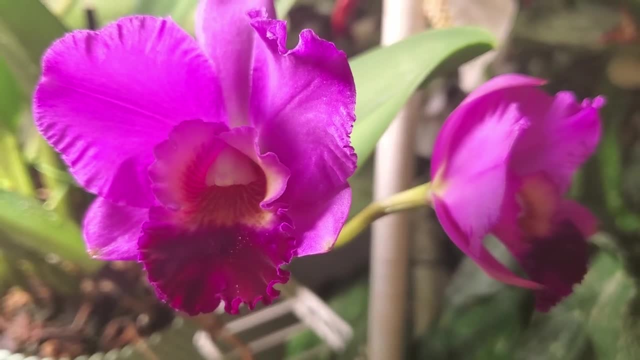 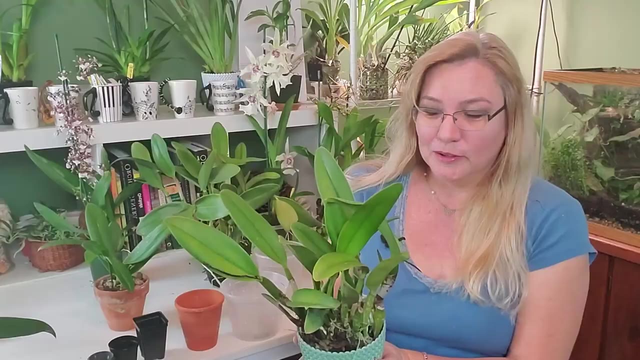 on doing. Usually they don't do this. Usually they just grow in one direction. but this one had some stress issues, decided that one side wasn't growing great, so it grew on the other side and the other side started growing and it just Once it got over its issues, it started growing on both sides again. So if I repot this, I don't need to. 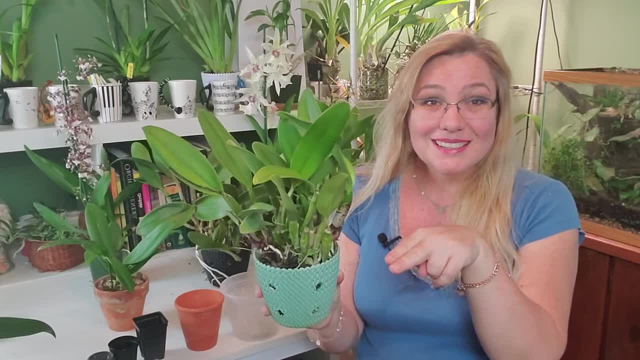 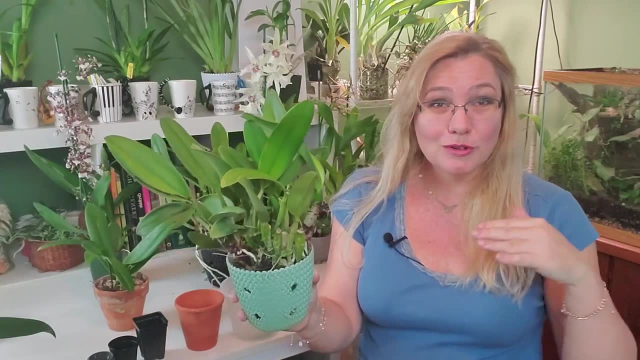 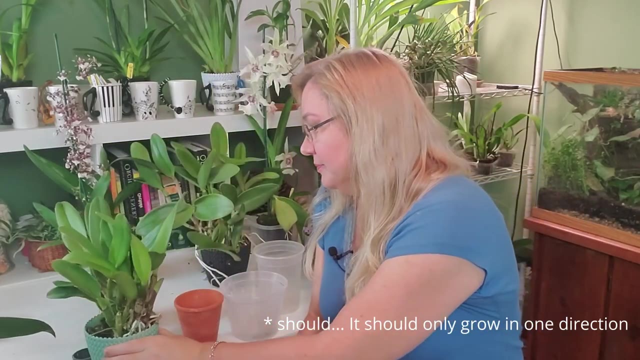 only think of: okay, two inches on this side. I need to think about also two inches on this side. Keep that in mind. which way is your orchid growing? If you have a sympodial orchid, it will only grow in one direction. I'll give you another example. The older growth started on this side and now it's. 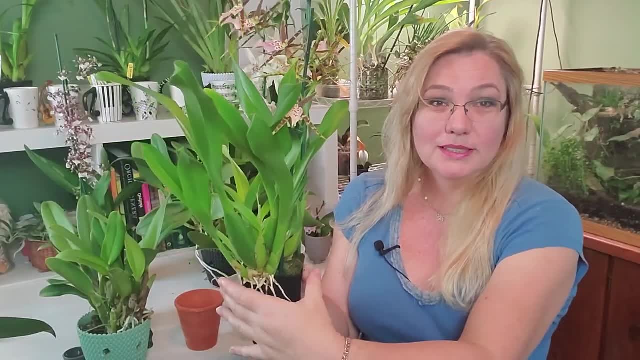 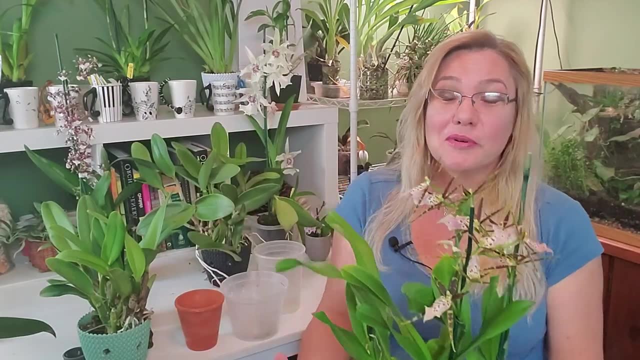 growing on this side. So if I repot this I don't need to only think of: okay, two inches on this side. It's growing outside of the pot on that side, So I need to calculate the size on this side. You know, add two inches here. Some orchids are just really slow growers, So you don't have to do all that. you know, over pot. Which brings me to a very important point, and that is: do not over pot. It's best if you under pot and keep that pot a little smaller than if you get a pot that is too big and just bury your orchid. So if you have a pot that is too big and just bury your orchid, You don't. 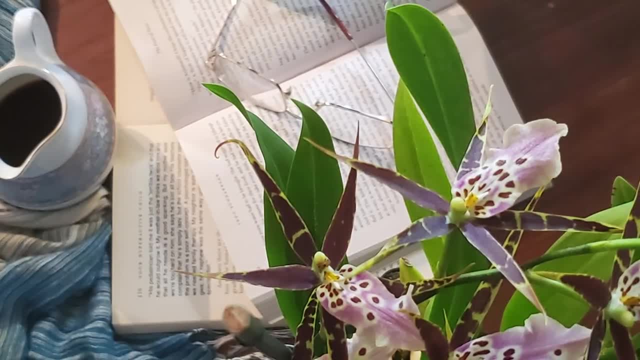 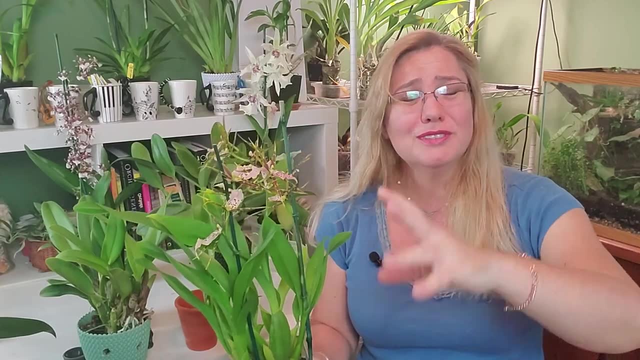 want to bury your orchid in there, And that is because of one thing: The orchid needs to feel stability. When you are about to repot an orchid, remember this is probably the second most stressful time of its life, And the first one was when you bought it and it came through transport. It had 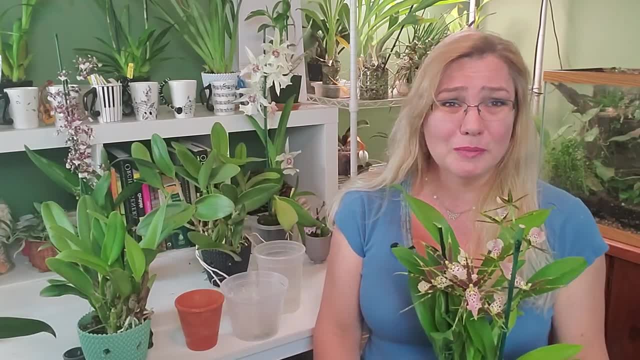 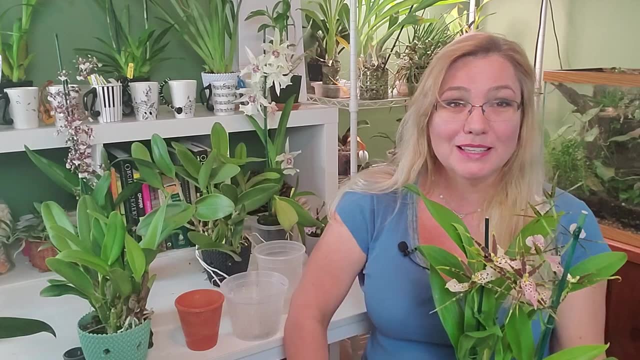 time to adjust to your environment. Now it's time to repot the poor thing. This is going to be horrible for the orchid. It's gonna hate it. It's gonna hate you for it. You know it's kind of like kids: You do what's best for them and they hate you for it. So forget that part. Make sure that they feel. 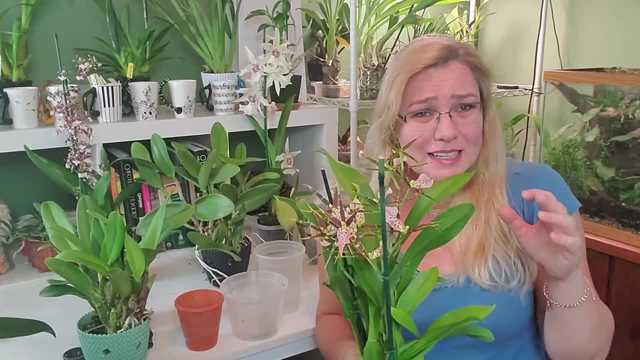 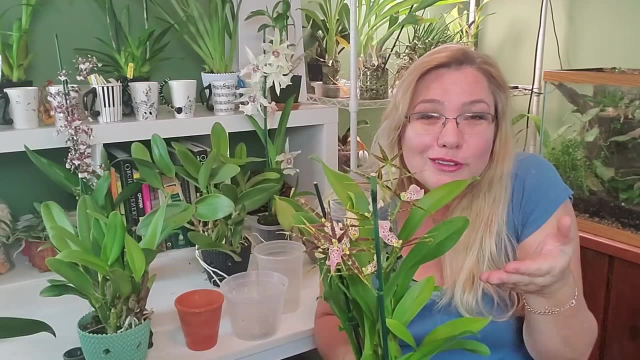 safe in their new pots. They need to feel cozy and warm. It's kind of like, you know, going back to little kids. It's kind of like putting them in bed. You want to, you know, make sure the little covers are all around there, You know, snug them in real nice and tight and make sure that they they feel. 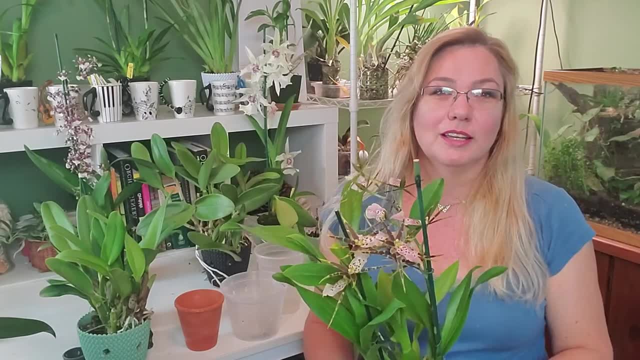 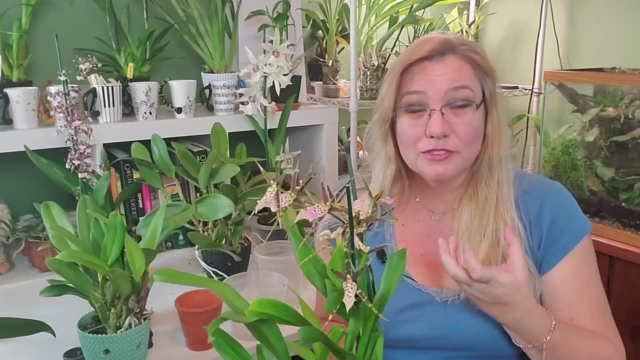 cozy and safe. Same thing for the orchid, So same thing for this guy. When I repot him, I need to get a pot that is going to make them feel safe, Make them feel secure, That is snug and tight and will allow them to repot. 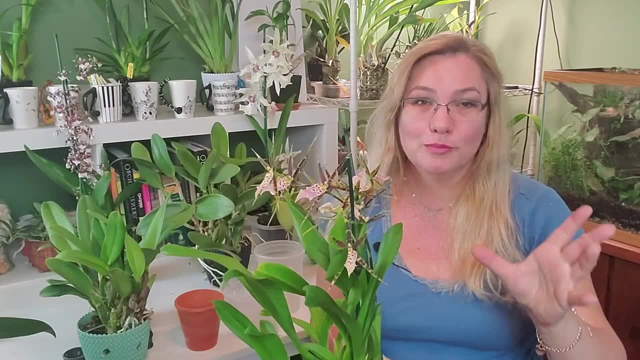 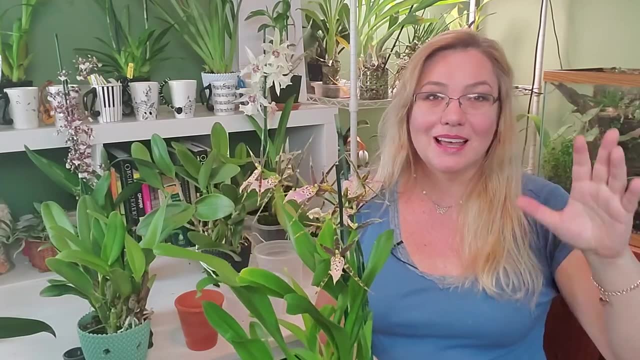 And still room to grow. So that's why we keep the one inch, 2.5 centimeters on a Phalaenopsis, And if you have a sympodial orchid- Oncidiums, Catlea, Dendrobiums, others- They will need a pot that is a. 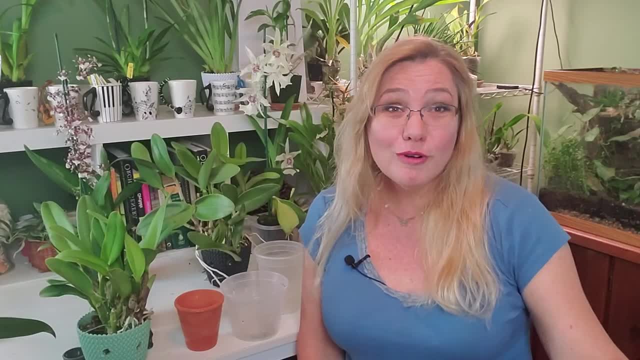 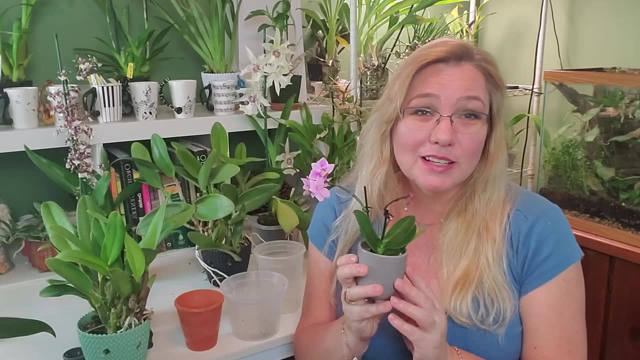 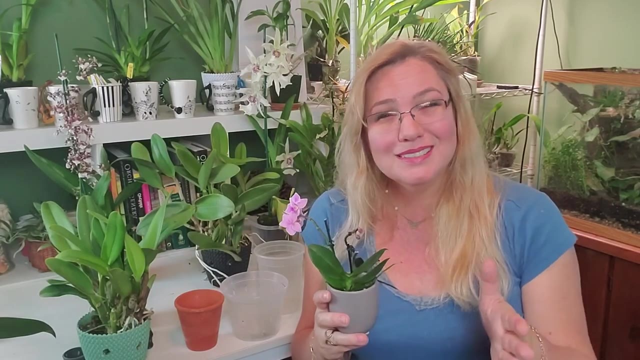 little wider on the sides And just like Grammar. there is an exception to that rule, which is a mini orchid. Now, mini orchid. when you repot this little guy, you will need a pot that is the exact same size, Because, even though he is small, that's the only size that he's ever going to get, So the roots aren't going to expand. 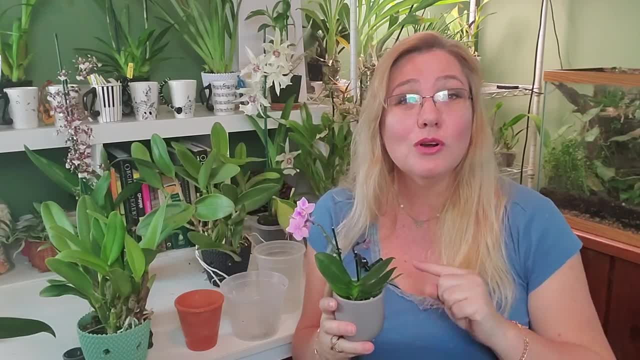 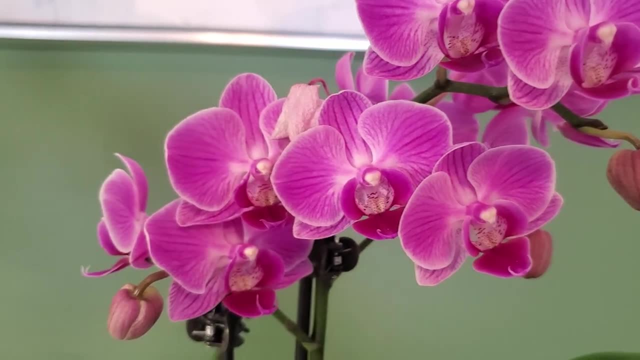 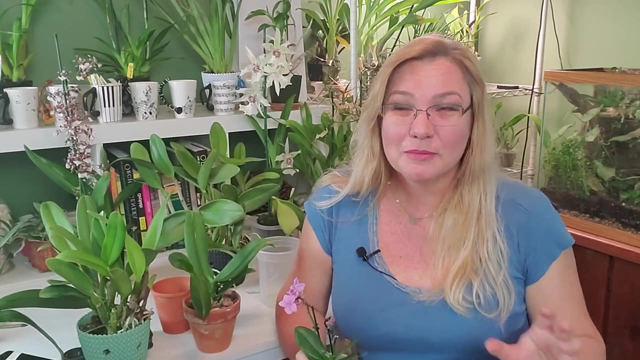 that much. So when you repot your mini orchid, you are going to use the same size pot, So miniatures keep the same size pot. That's the exception, and we can go on to our next point. By the way, if this video is helping you in any way of clarifying some kind of doubt you have, please give it a like or. 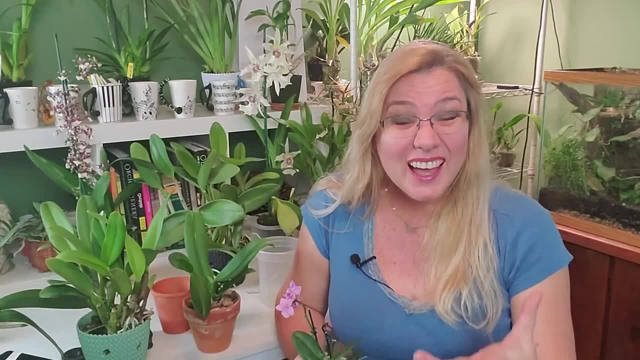 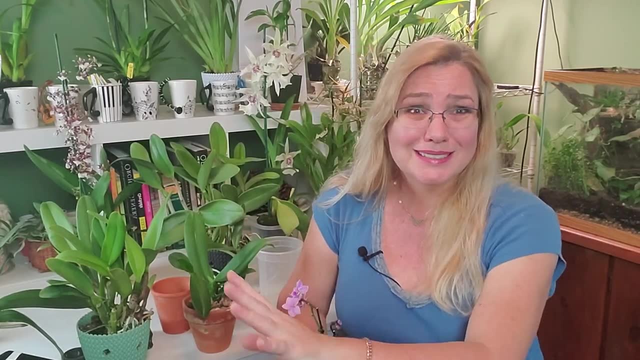 comment or tell me what I'm doing wrong, Because that actually helps me to know what videos to do more of or what videos to stay away from. You're like never more. this topic sucks, So please give it a like or any kind of feedback is what I'm. 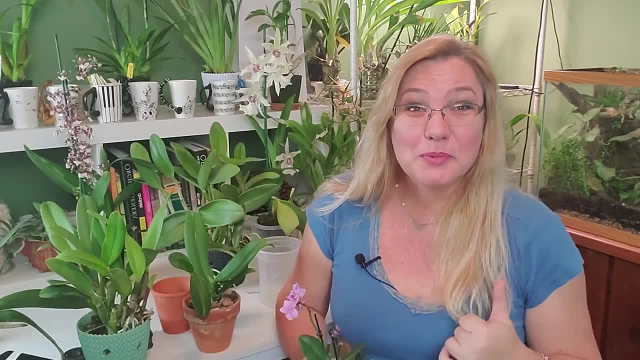 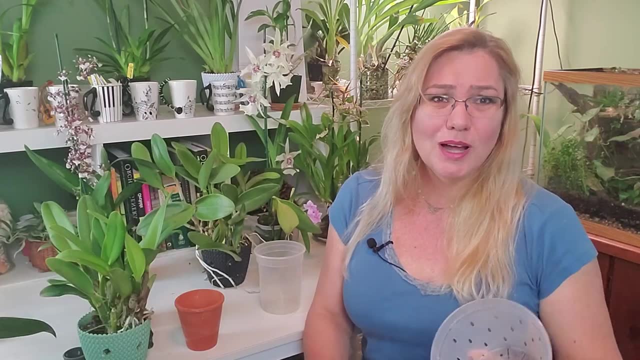 asking for really Okay, let's go on to the next point. The second tip is: does it matter if my orchid pot has holes in it or not? Do I really need to put holes in it? And I would answer this If you. 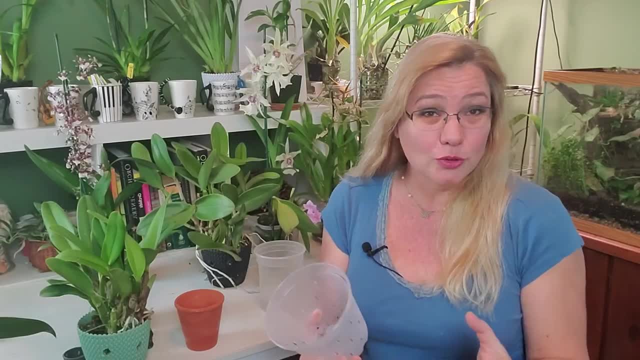 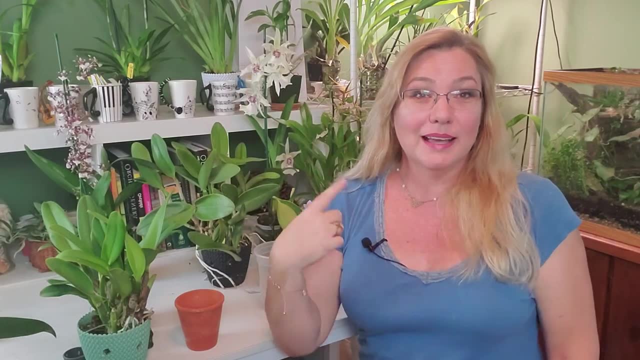 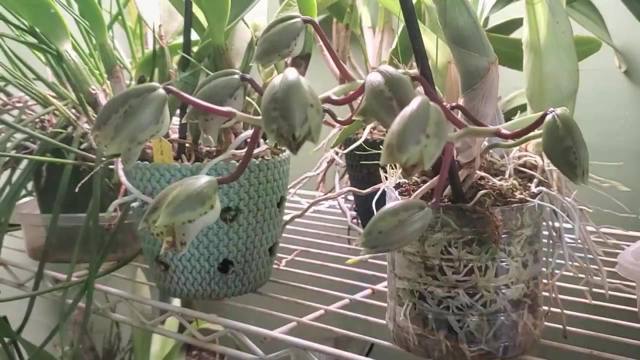 have an orchid that is so used to humidity, or you have a terrestrial orchid or a semi-terrestrial orchid, it will not need that many holes in it. For example, the catasetum pot which is right there- I'll zoom in- It only has holes on the bottom third of the pot, because the rest, those roots really love. 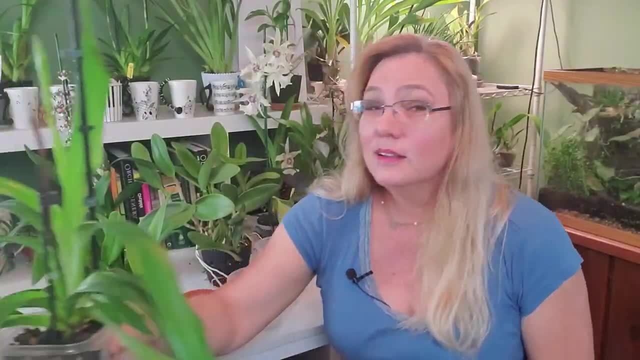 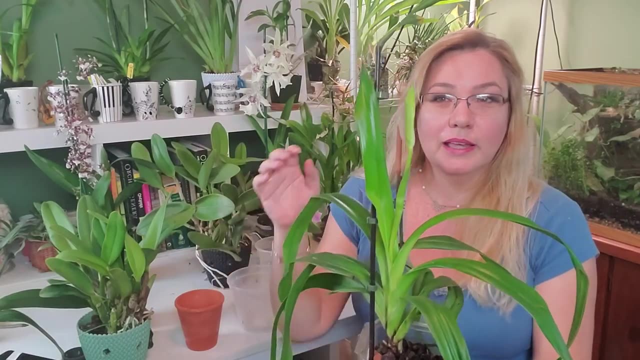 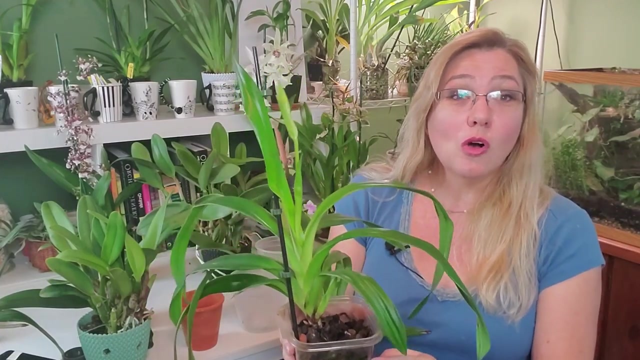 that water, So I need to keep that humidity high. Another orchid is a- oh, I gotta take this off. Another orchid is a pathiopedilum, and this one is putting out a new spike and also a new growth on this side. There are no holes in this pot. There is nothing on the drainage holes, of course. 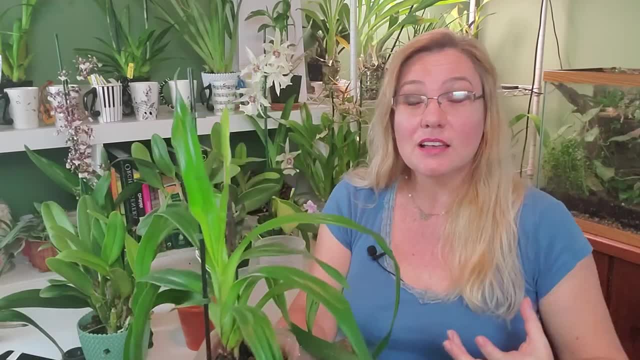 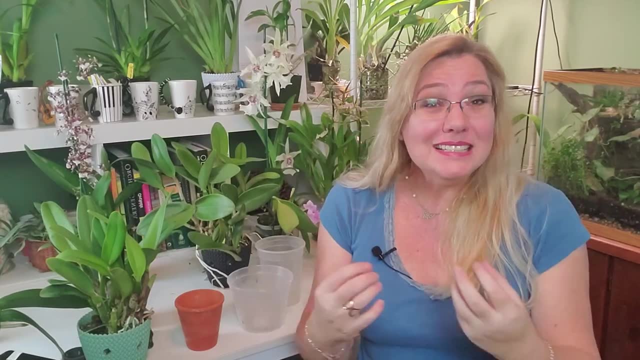 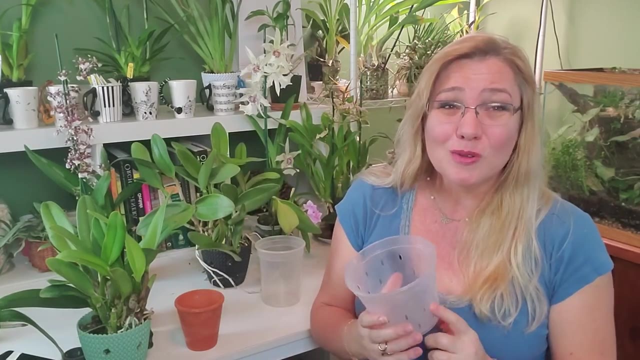 There are no air holes on the side of this pot because it loves that humidity, Since my home office is so dry- I mean so dry- So I need to keep that humidity really high around that pot, So you do not need holes. but if you're just starting out, yes, get holes in that pot. Now you can make. 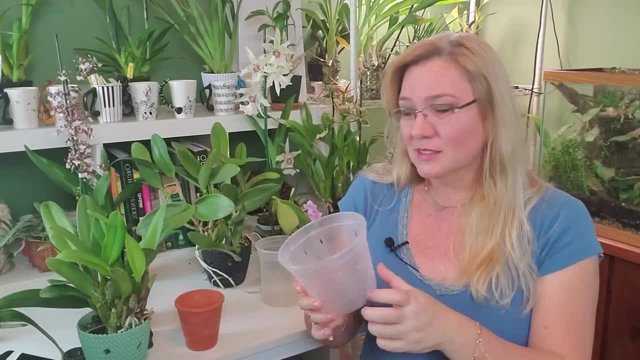 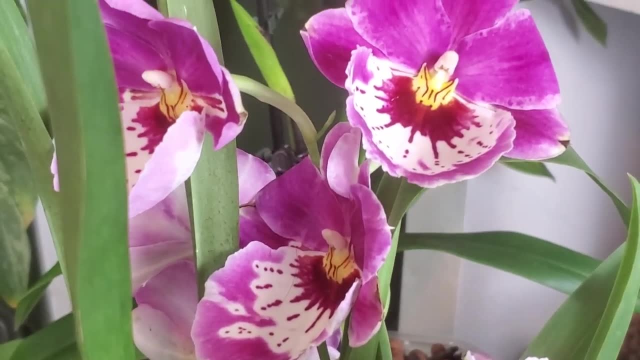 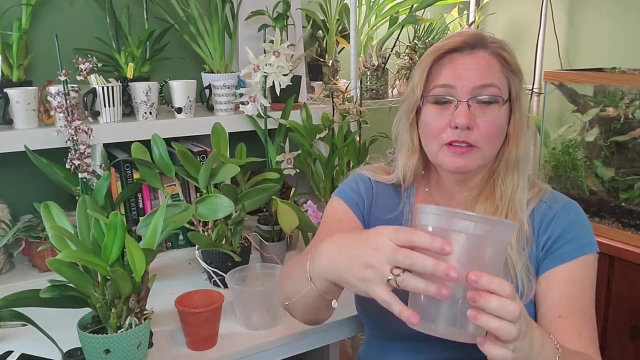 holes by either heating up scissors and getting a normal plastic pot like this- Heating up scissors, heating up a hot iron, getting a hot nail. Usually, if you try scissors, you're going to bust your pot like that, which is normal. That's just part of the learning curve. Don't worry about it. You can use. 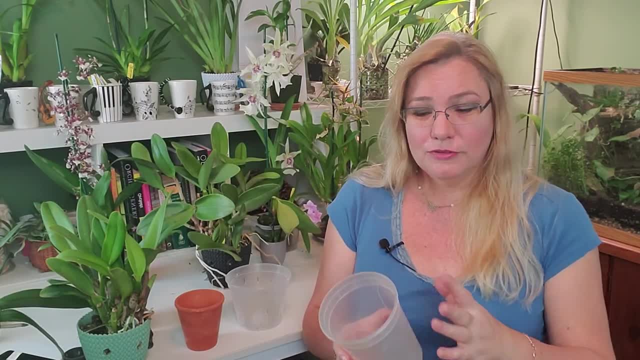 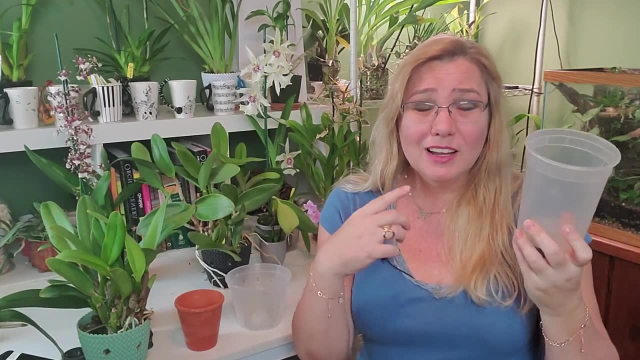 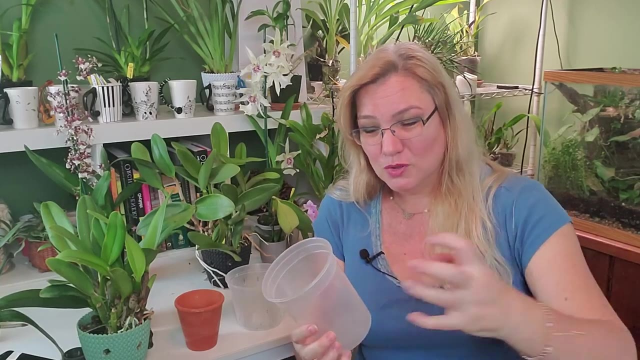 it. It looks horrible, Just make a whole bunch of holes. So, for example, if I use only sphagnum moss, I would never use a pot with no holes in it. I want those holes because sphagnum absorbs so much water. Sphagnum is like a sponge, so it's going to absorb everything around that. If I only have inorganic 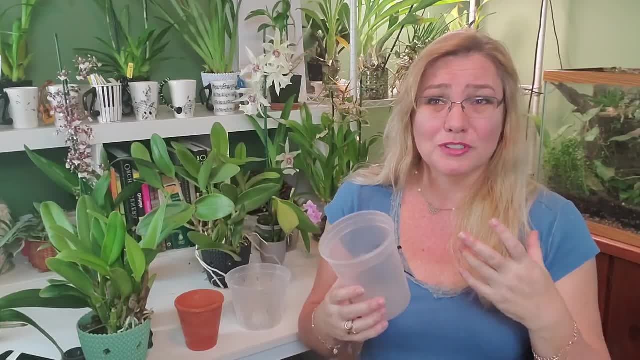 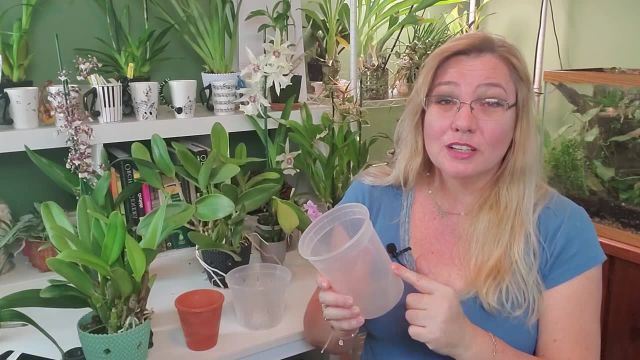 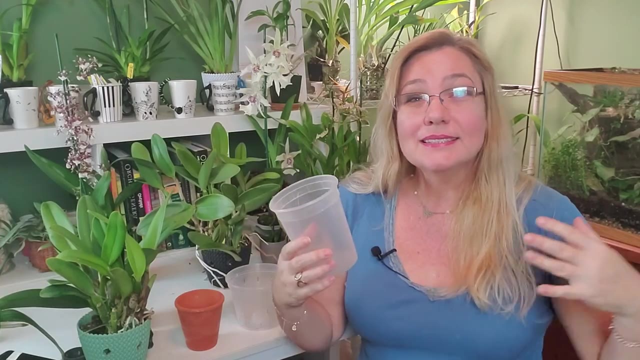 material kind of like river rock or pebbles or charcoal, will absorb it, or just orchid bark in there. I can use a pot without any holes because it's not going to absorb that much. So the whole idea of having holes in your pot is to get that air in and out and to make sure that there is. 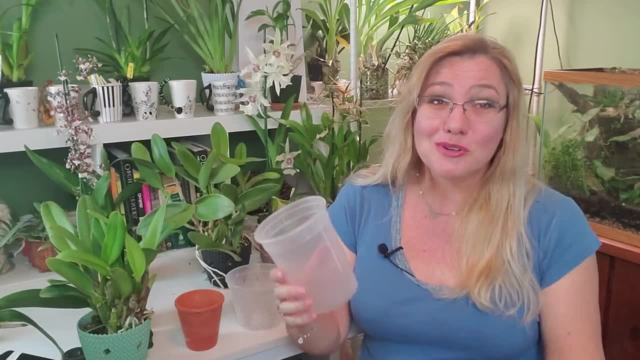 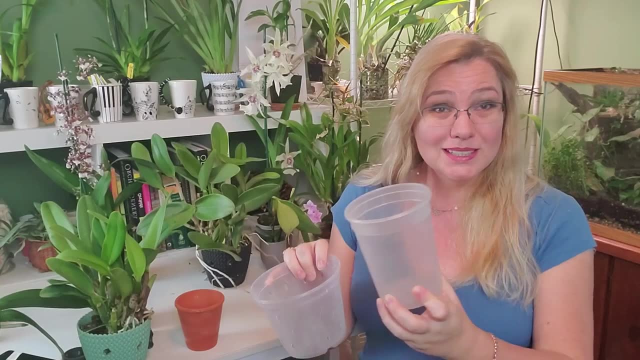 ventilation. Once you understand and get a hang of it, you don't need to buy those expensive pots anymore because honestly, these are pretty expensive. Just get an old pot, make holes in it somehow, and even if they're not, you can make holes, You can make slits, You can use. 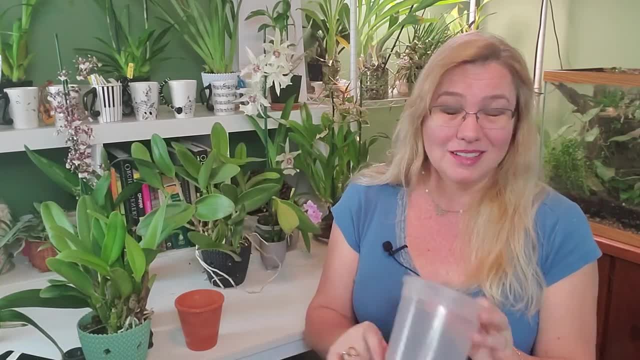 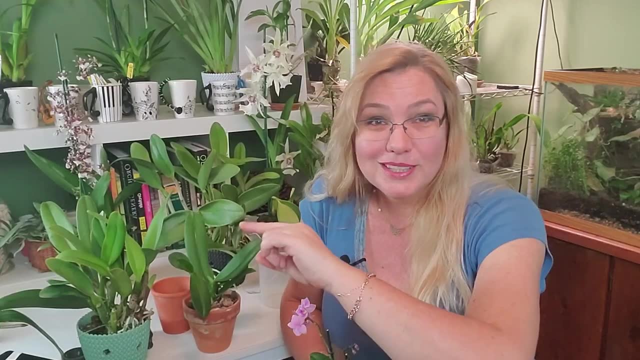 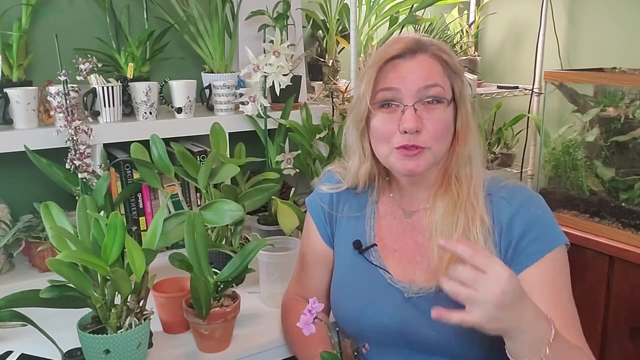 any kind of thing just to get ventilation in there. It doesn't have to be pretty, because the pretty part is on top. I do want to take a parenthesis out here before I get to the next point, which is: thank you so much. I put my first poll out on my community. You can go to my page. 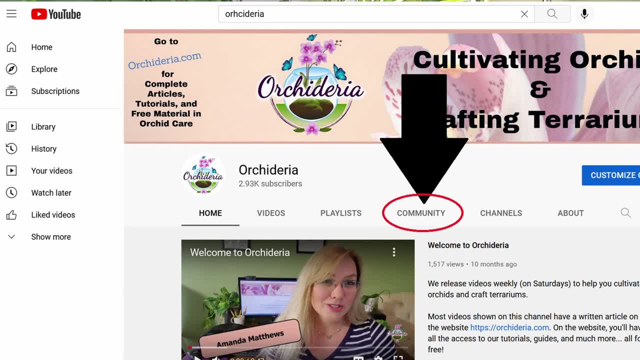 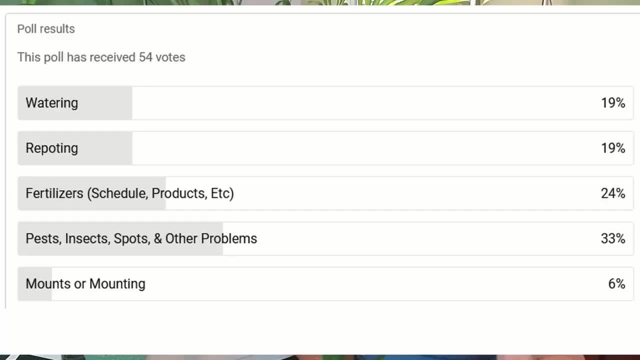 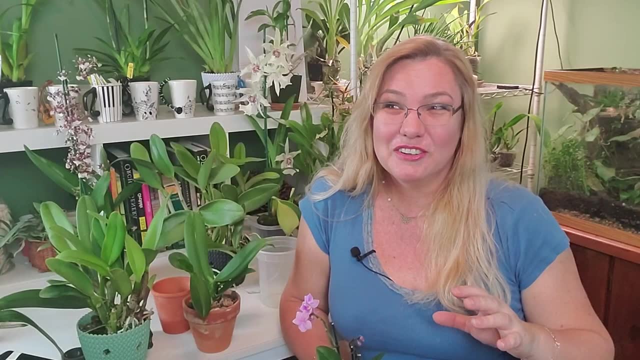 and look on the community and I put out my first poll of what topics you would like to see more of, and I got an amazing response. I thought, well, nobody's gonna answer, But you guys did so. thank you so much for that. and I found myself going back to it every, every like. 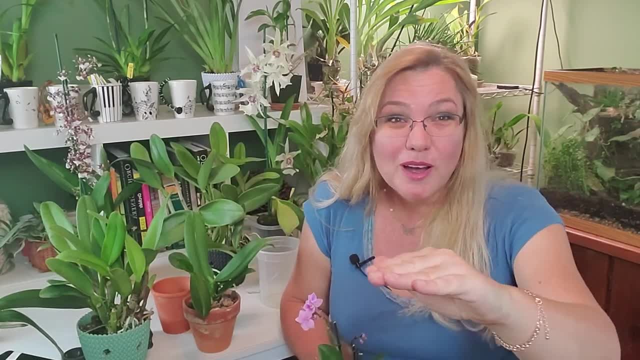 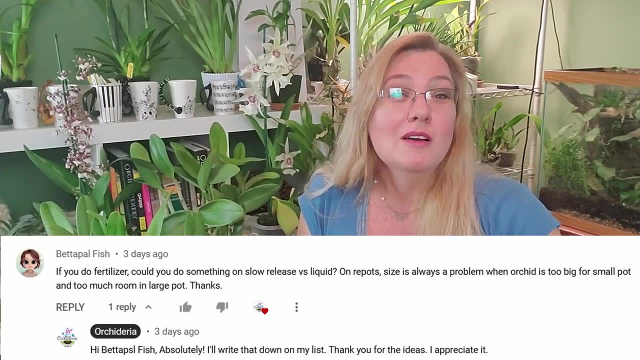 30 minutes like, okay, what? what's the answer now? and I receive: like repottings growing. The next one: oh it's, it's pests and spots and problems and oh no, it's mountain. This video was an answer to that, because I want to thank you so much. Better, Pal Fish, You took the time to to write out and 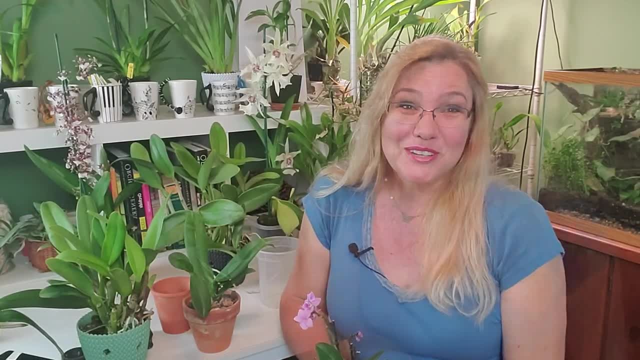 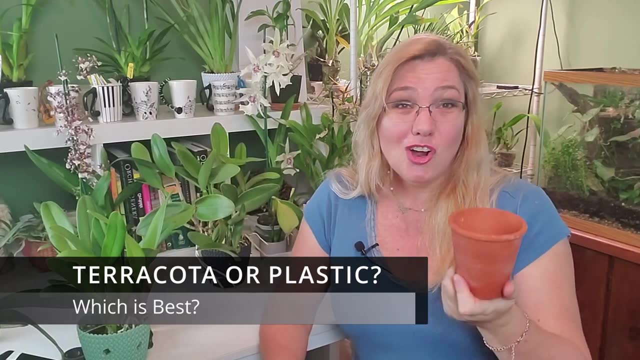 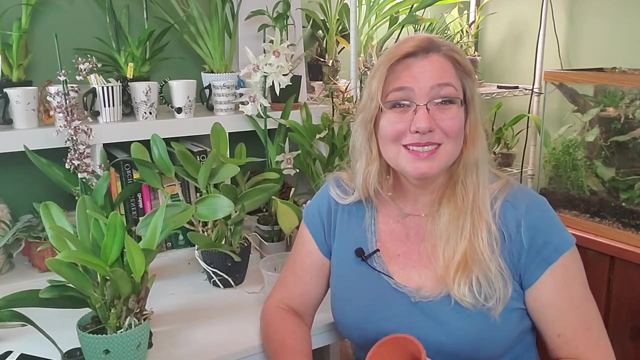 tell me what you wanted. So this is for you. The next question: Do you like terracotta or plastic? which is best? There are great advantages to using a terracotta or a clay pot, And the biggest problem I found with these is trying to get the holes in them. Have you tried, Honestly, have you tried, to drill a hole in these? 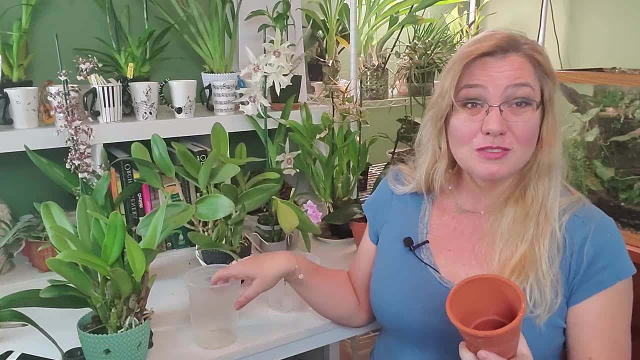 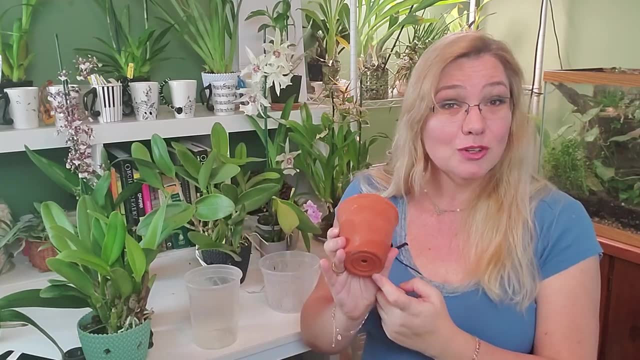 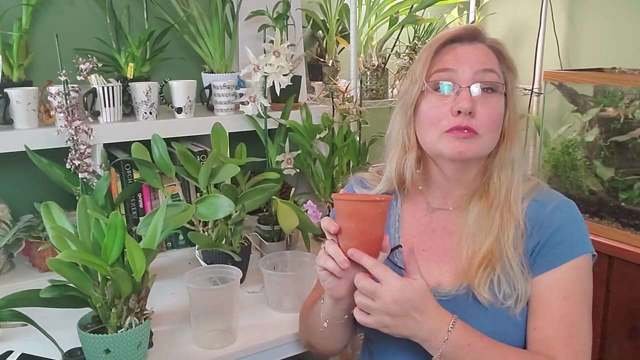 I mean that. talk about manpower, talk about using your muscles and working out. I managed to break like four, four of these until I gave up. There is one drainage hole at the bottom, but now here's the good part. there are advantages to these. these will keep the roots cooler. so if you live in 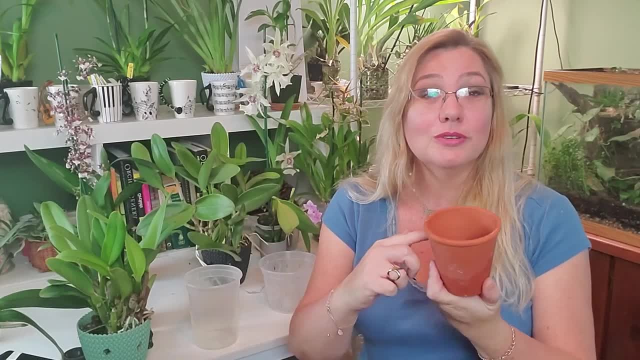 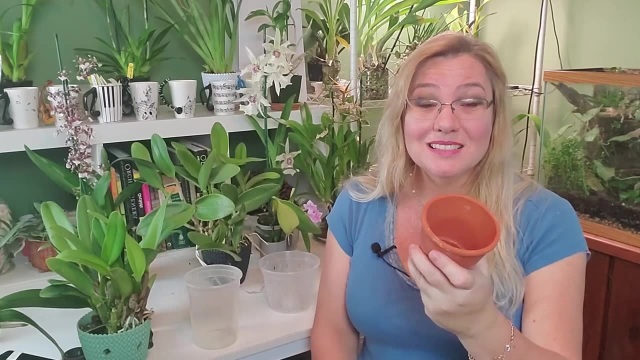 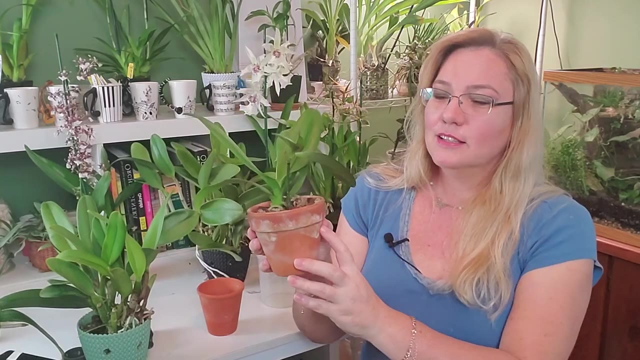 a hot environment. these are perfect because they will keep the roots cooler and in that temperature range that is more adequate for them, and they will also absorb tons of moisture, which makes them pretty ugly over time. for example, this guy right here has been in terracotta and yeah and ignore. 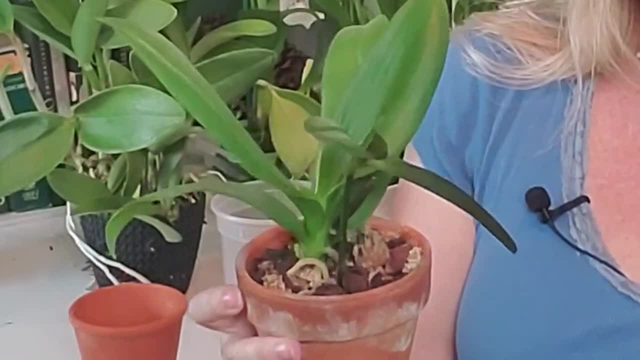 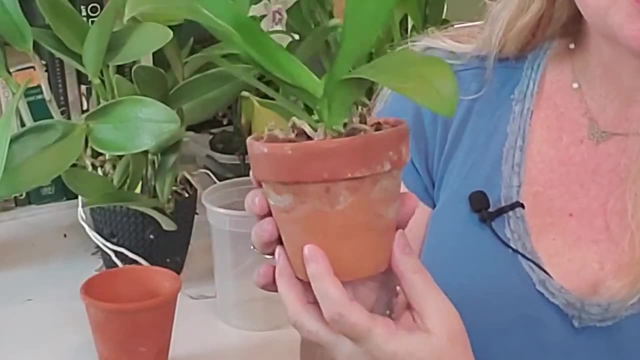 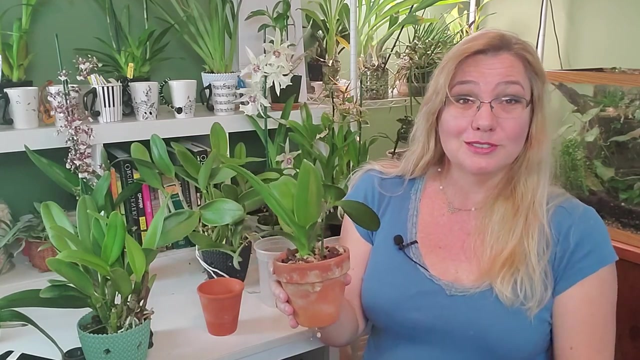 this cakey here. um, he broke off. yeah, just ignore him. um, look at the bigger one. look at the mama plant. it turns out to be pretty ugly over time. but if you can ignore this, please do, because it is a great solution and you will have to water a little bit less. this pot will absorb a lot of. 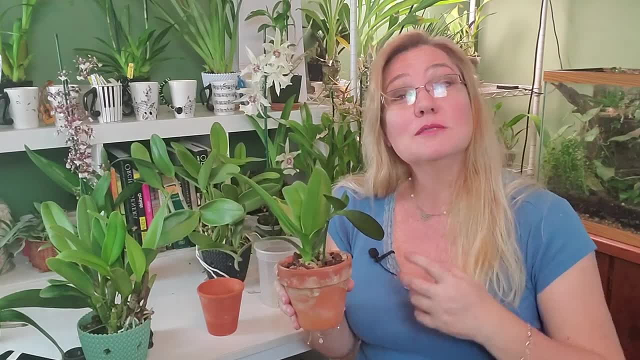 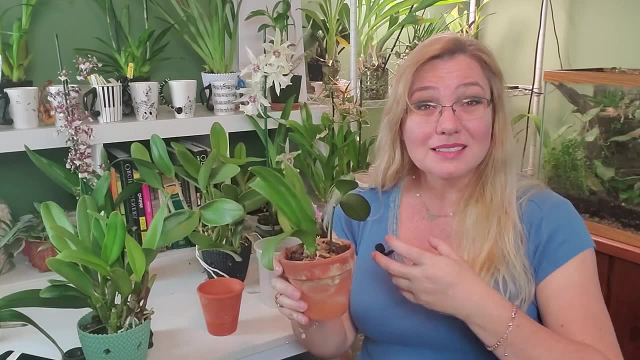 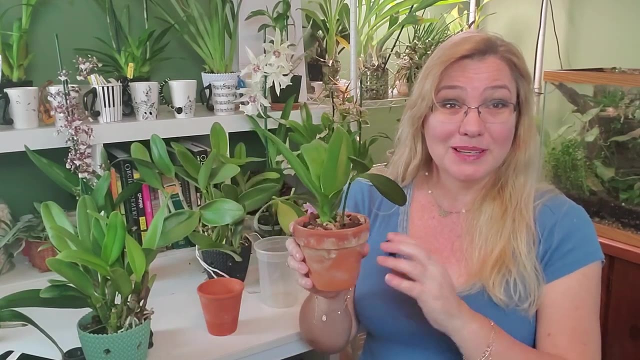 water. now, a good thing about this is this: this pot is breathable, so you really don't need the holes. i mean it doesn't look like it, but it actually does provide for air to come in and out of this pot, so that is an excellent idea, for this is my second runner up, my second choice of. 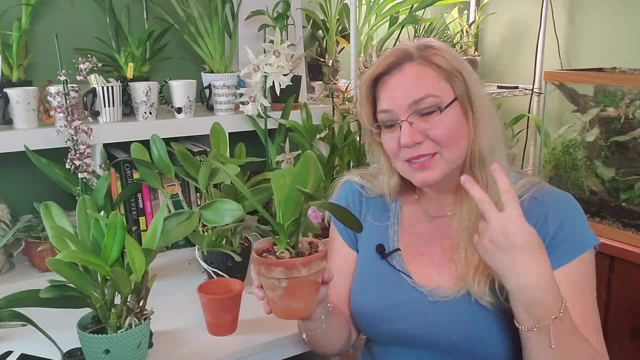 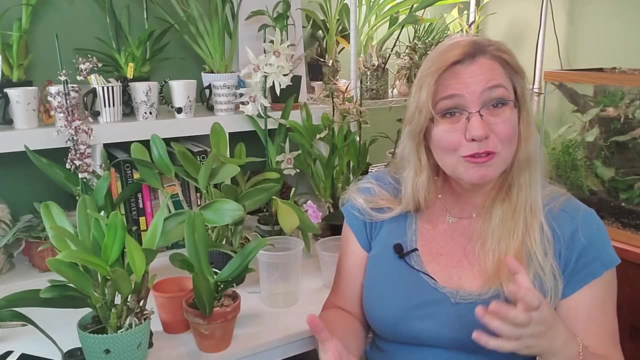 what pot to choose. but first is plastic with holes, the second is a terracotta pot. the third runner up would be to mount the orchid in a little wooden basket or some kind of basket, or mounted on a log or a tree or something to get that mounted. 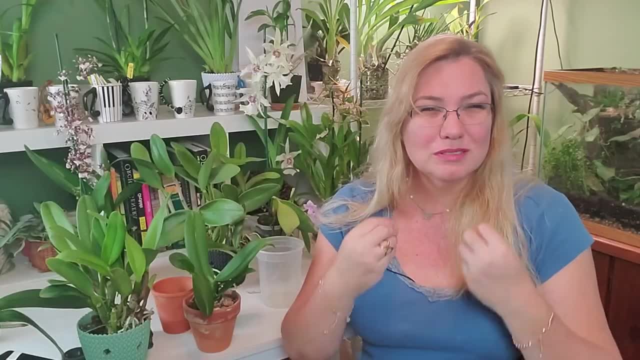 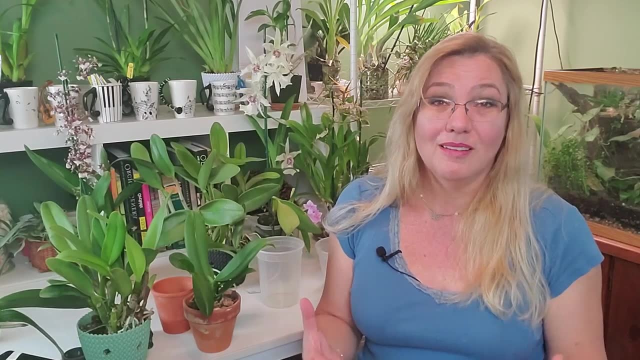 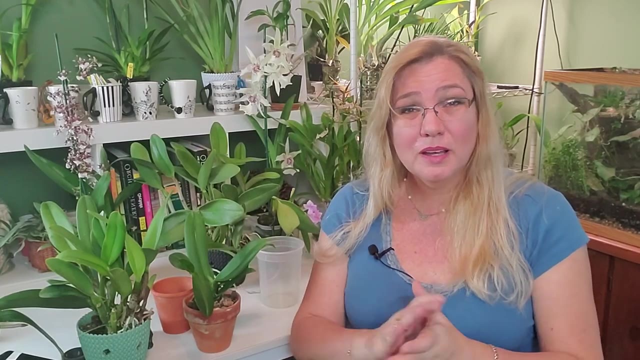 keeping these orchid roots dry and wet is really really hard and to get that balance. but if you have a very humid environment it's great to mount them. if you have a drier environment, mounting can be a little tricky, so keep that in mind. with the third kind of pot, which would 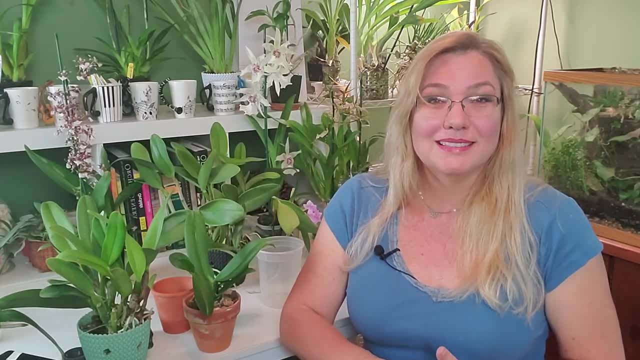 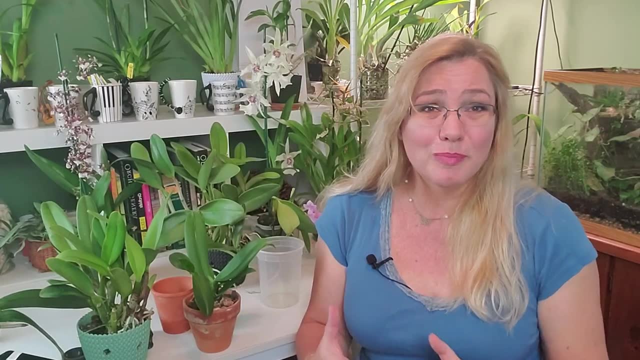 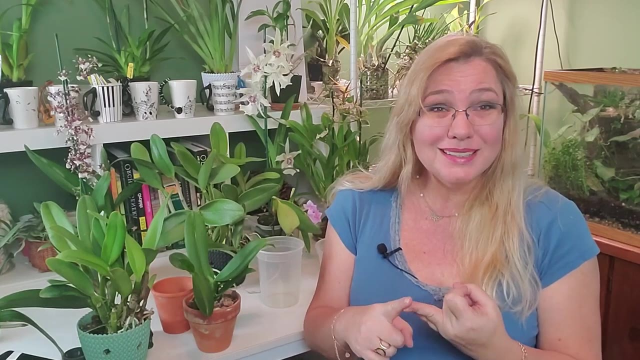 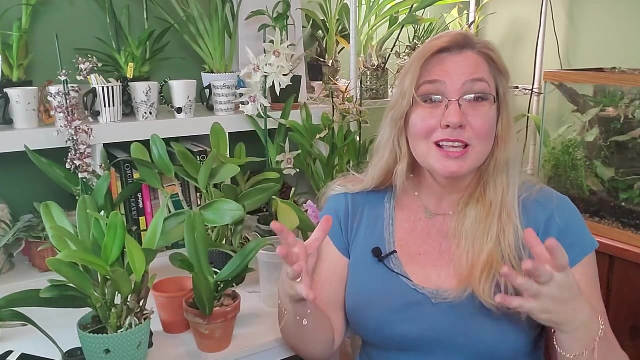 be a basket to plant. keep your orchids in. what nobody talks about, though, is this the most important thing about choosing the pot. really isn't the size, because your orchid will forgive you. um. it really isn't the plastic or terracotta, or ceramic or whatever. it really isn't that it's. 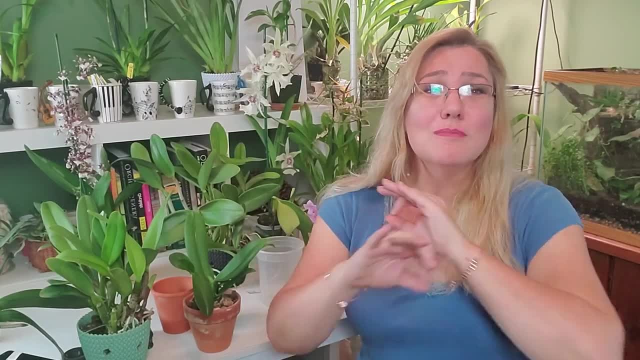 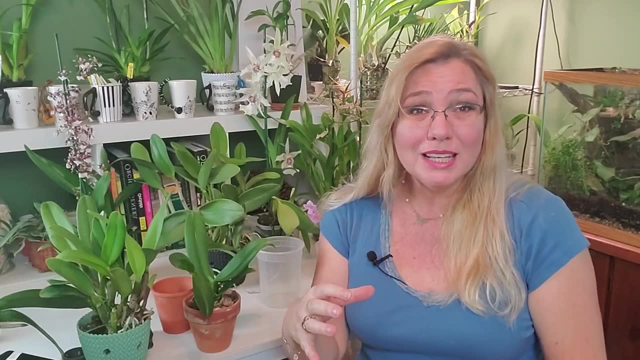 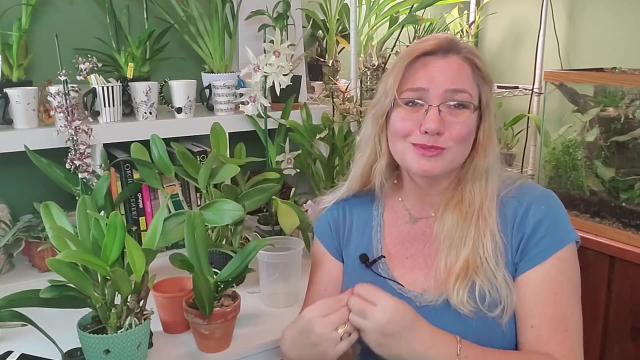 drainage, drainage, drainage, drainage: that is the most important thing about selecting the right type of pot. so if you have a pot and it's not draining, that's going to kill your orchid, whether it's plastic, terracotta, ceramic or anything. so don't, don't, don't, don't get a pot. 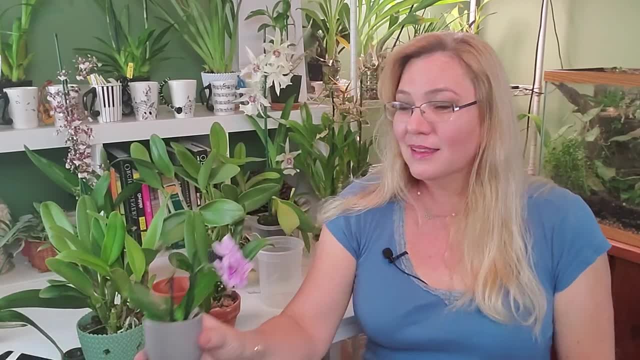 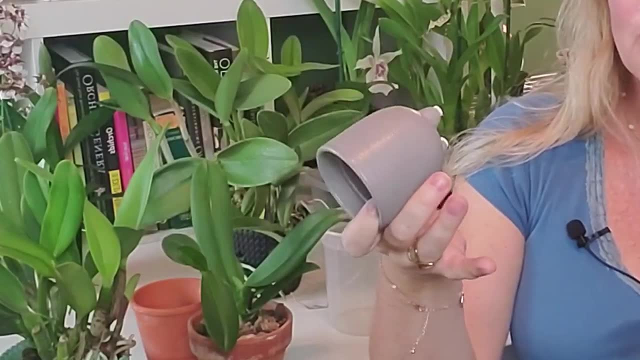 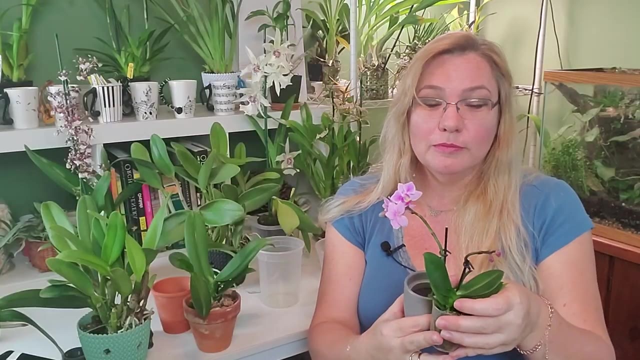 that doesn't have drainage, for example. this is cute, I love this pot. let me take them out here. I love this pot, but it's horrible. there are no drainage holes. this is a sticker. there are no drainage holes. so even though I love my little mini and I put him here when he's flowering, when 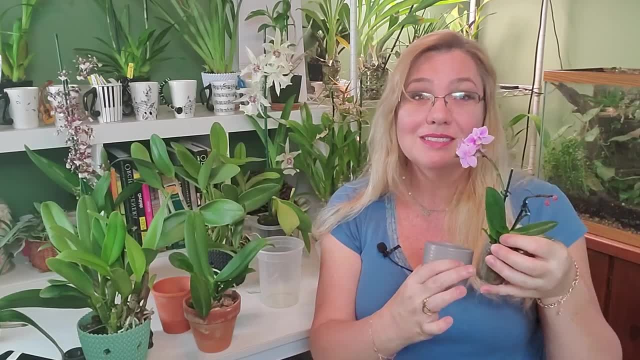 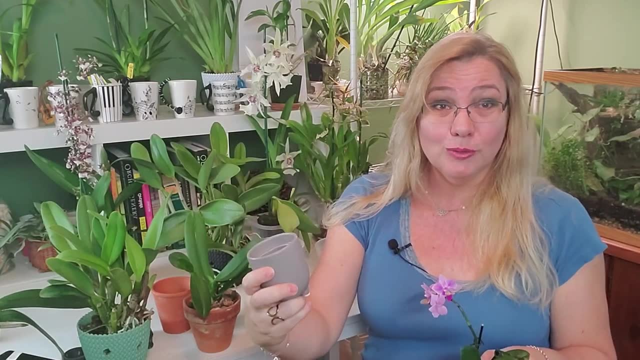 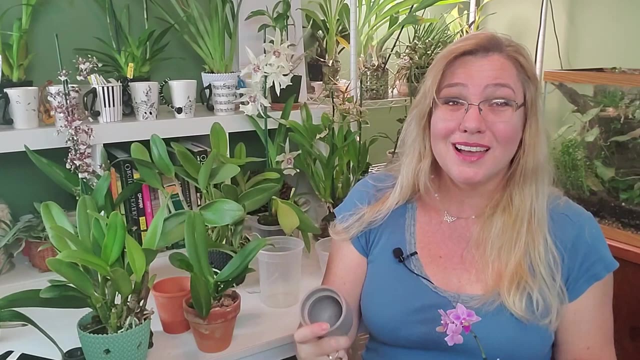 he's not flowering. I take him out and put him on my shelf and there's the little plastic pot that he has in. this is only good for showcasing your orchids that are in bloom. when they're not in bloom, get them out of this pot. this is a decorative pot. decorative pots do not do anything. I mean they trap the air. they trap the.